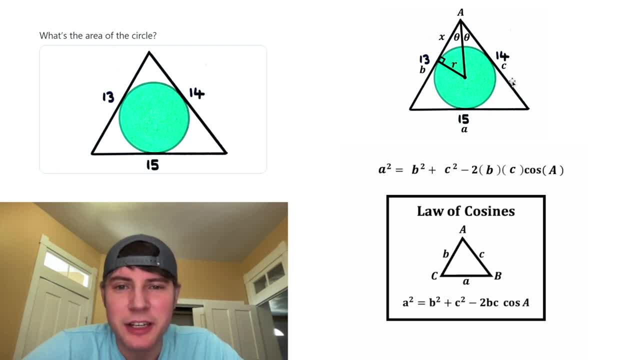 capital A, and then these two sides, b and c. we can now use this formula: Lowercase a is equal to 15.. Lowercase b is equal to 13, so we can change both of these b's into 13.. And then lowercase c. 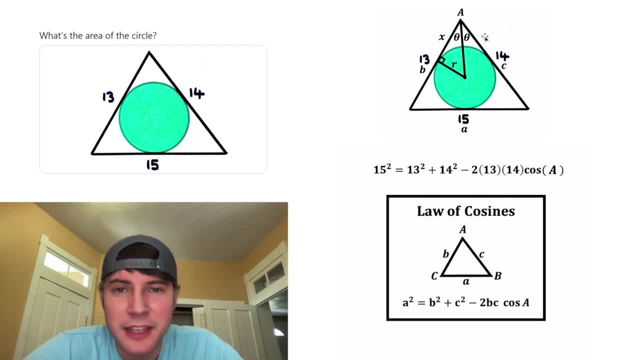 is 14,, so we can change both of these c's into 14.. And then the angle a is this entire angle up here, so it's going to be 2 theta. And now let's clean things up: 15 squared is 225.. 13 squared is: 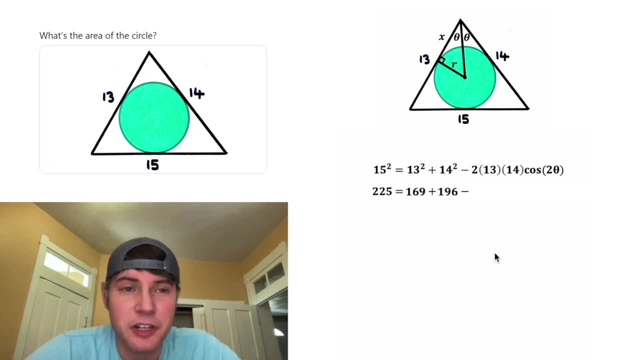 169.. 14 squared is 196.. And then we're going to subtract 2 times 13, times 14, which is 364, times cosine 2 theta, And then 169 plus 196 is equal to 365.. We can subtract 365 from both sides. 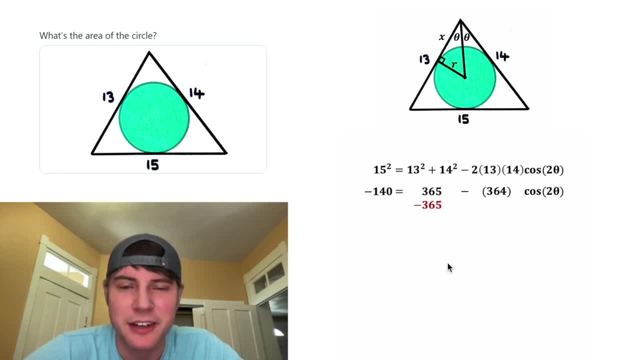 On the left-hand side, 225 minus 365 is equal to negative 140.. And on the right-hand side, these 365s will cancel each other out, And then we can smoosh everything together. Next, let's divide both sides by negative 364.. Negative 140 over negative 364 is equal to 5 13ths. And then 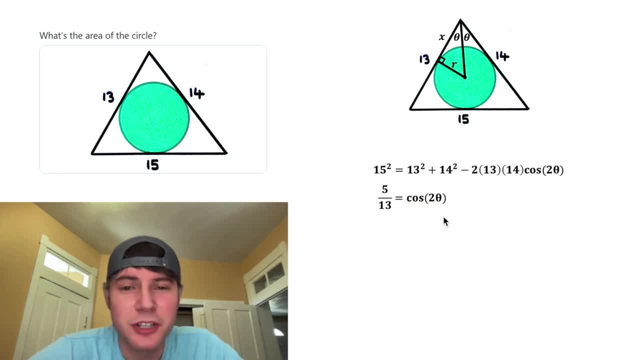 these negative 364s cancel each other out. So now we have cosine of 2 theta is equal to 5 13ths. It's tricky to work with this double angle, so we're going to use the double angle formula to get rid of the double angle. It tells us that cosine of 2 theta is equal to 2 cosine squared. 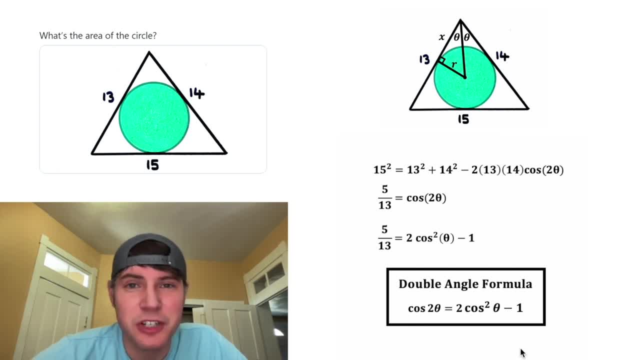 theta minus 1.. It's pretty cool to see how these notes are derived. We just don't have time to do it right now, And then from here we can add 1 to both sides. On the right-hand side, the negative 1 and the positive 1 will cancel each other out. 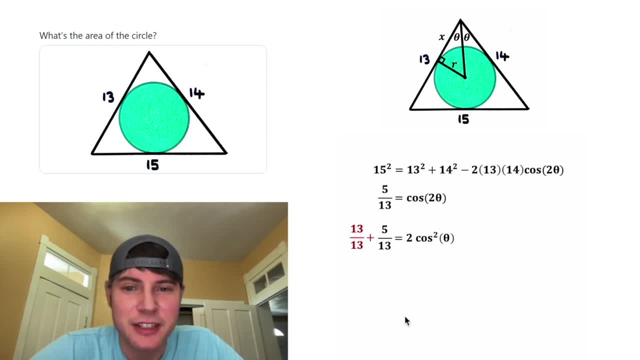 And on the left-hand side. this 1 can be rewritten as 13 13ths, And 13 13ths plus 5 13ths is 18 13ths. Next, we can get rid of this 2. We can multiply both sides by 1 half. On the left-hand side. 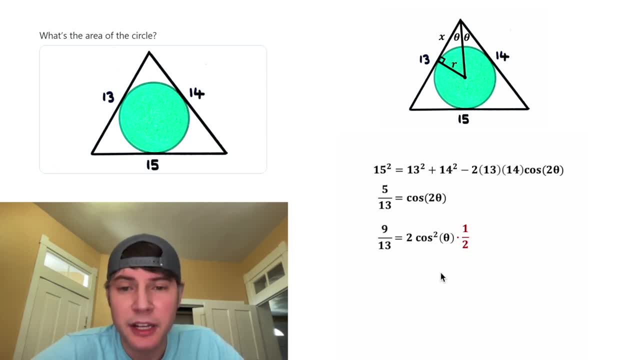 this 1 half is going to change the 18 into a 9. And on the right-hand side, the 1 half and the 2 will cancel each other out. So we have the cosine squared. theta is equal to 9 13ths. 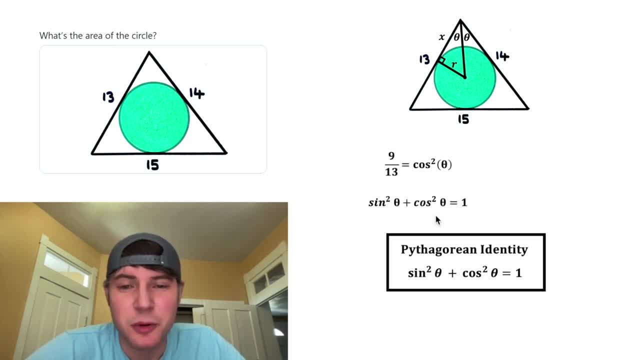 Next, we can use the Pythagorean identity. Sine squared theta plus cosine squared theta is equal to 1.. This one's also pretty cool to derive. I think I've made two videos on this. We know that cosine squared theta is equal to 9 13ths, so let's substitute that in And we can. 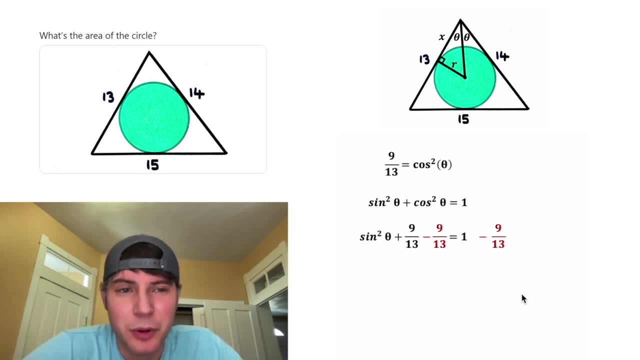 bring down everything else. Next, we can subtract 9 13ths from both sides of the equation. On the left-hand side, the positive 9 13ths and negative 9 13ths will cancel each other out, And on the 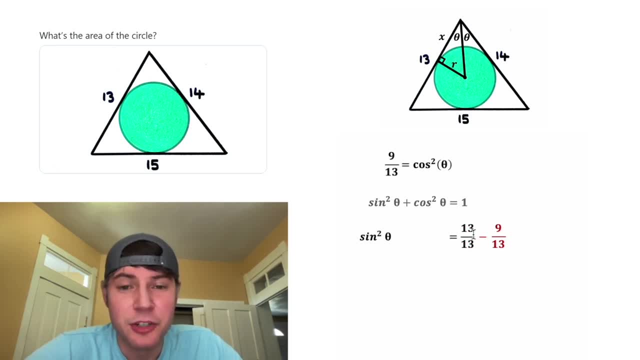 right-hand side. we can make this: 1 13 over 13ths, And 13 13ths minus 9 13ths is equal to 4 13ths. So now we have cosine squared theta and sine squared theta. Let's square root. 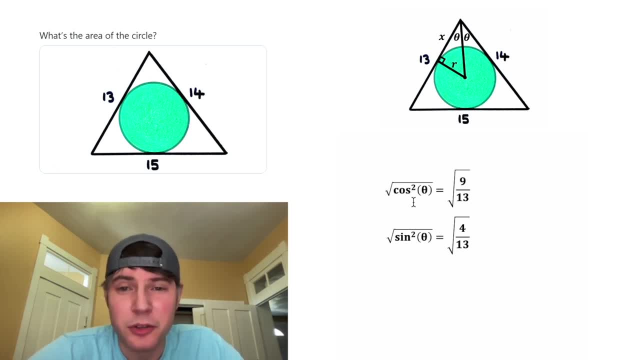 both sides of both equations. On the left-hand side, the square root of cosine squared theta is just cosine theta, And on the right-hand side, the square root of 9 13ths ends up being the square root of 9 over square root of 13. And the square root of 9 is equal to 3.. And then for this: 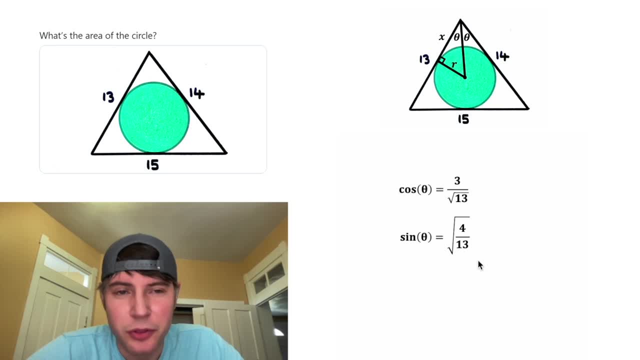 equation on the left-hand side. this is sine theta, And the square root of 4 13ths splits up into square root of 4 over square root of 13. And the square root of 4 is equal to 2.. So now we have: 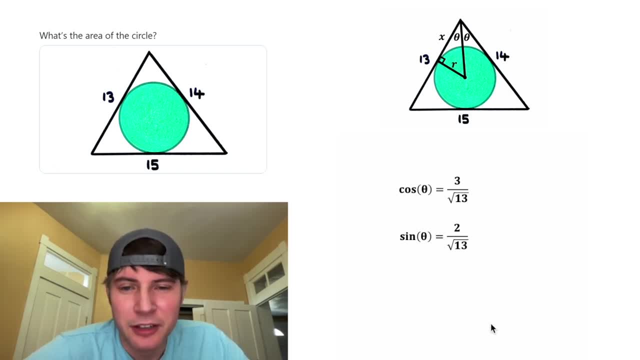 cosine theta and sine theta. And there's one more fun thing we can do. On the left-hand side, I want to divide this sine theta by cosine theta, which means on the right hand side we'll have to divide this by this. On the left hand side, let's rewrite this as sine theta over cosine theta And then on. 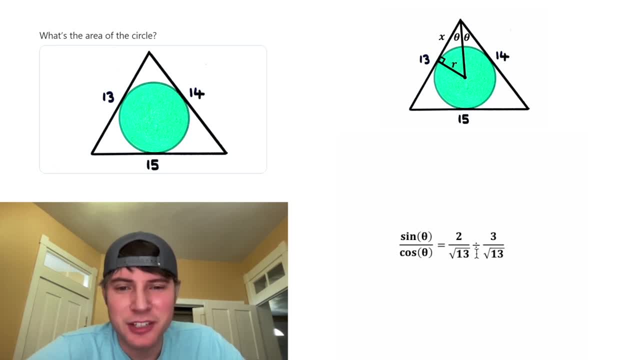 the right hand side, we're dividing fractions. A neat way to divide fractions is to change the divide to a multiply and flip the second fraction. Now we can cross, cancel This square root of 13, and this square root of 13 will cancel each other out, And so we're left with two thirds. And now we 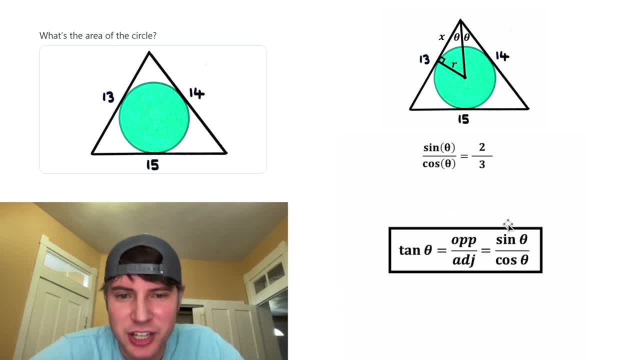 can use our notes for tangent of theta. So these notes are telling us we can change sine theta over cosine theta into tangent of theta. But these notes are also telling us the tangent of theta is equal to the opposite over adjacent. So now we're ready to go back to our original triangle. 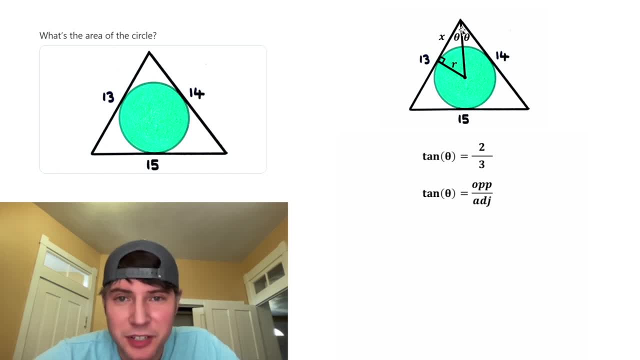 First we need to find the opposite of this angle, theta. Well, the opposite of this theta is equal to r, So we can change the opposite into an r. And then the adjacent to this angle is the x, so we can change adjacent to x. So we now know, the tangent of theta is equal to two thirds. 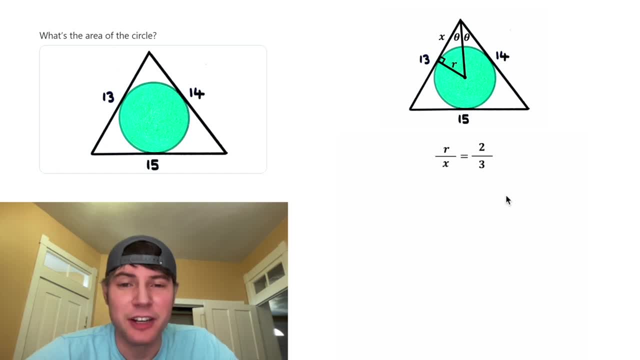 but it's also equal to r over x, So we can set r over x, equal to two thirds, And this looks important. so let's put a box around it, And now we can bring back our notes for the tangent lines, Since these are both tangent lines that meet at a. 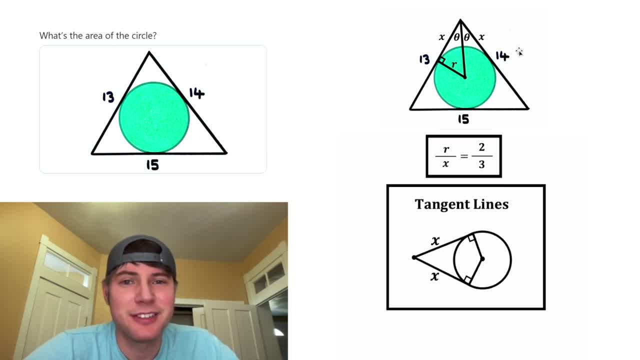 point. we know this piece is also equal to X. Now let's look at this side of the triangle. If the whole side is equal to 13 and this piece is equal to X, that means this piece will equal 13 minus X. Now looking again at our tangent notes.